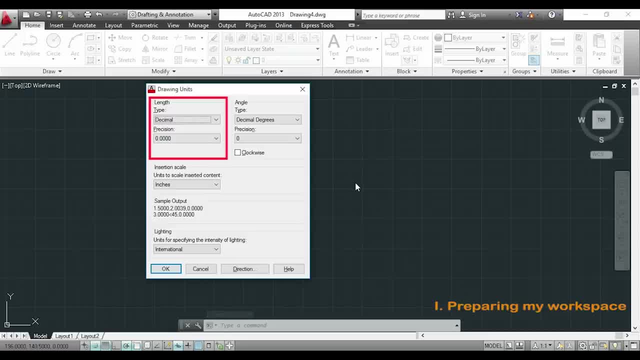 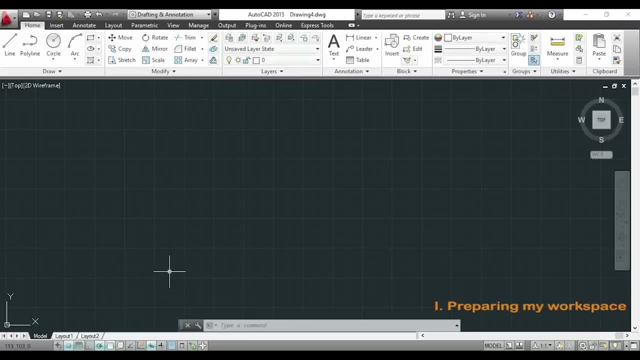 Here, where says length. I have to choose the type of measurements that I need and the precision that I want. In my case, I will use decimal and precision zero. For the units, I will use millimeters. Now I click OK. 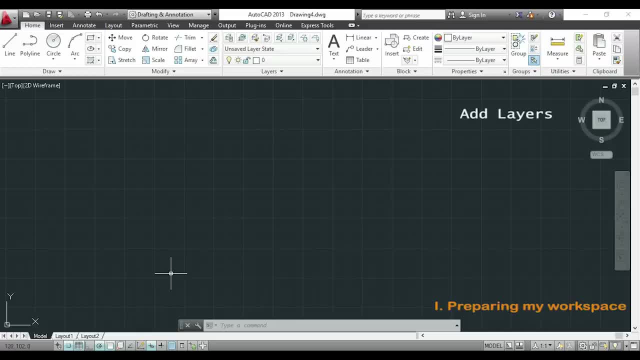 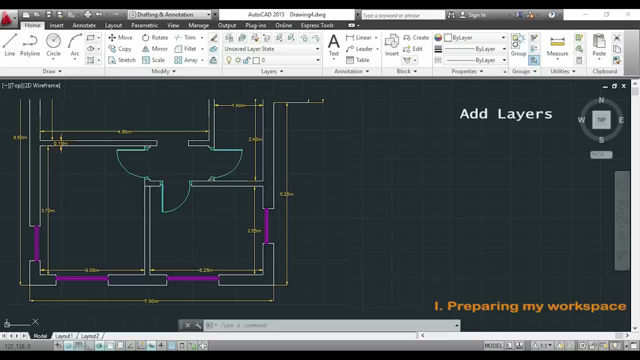 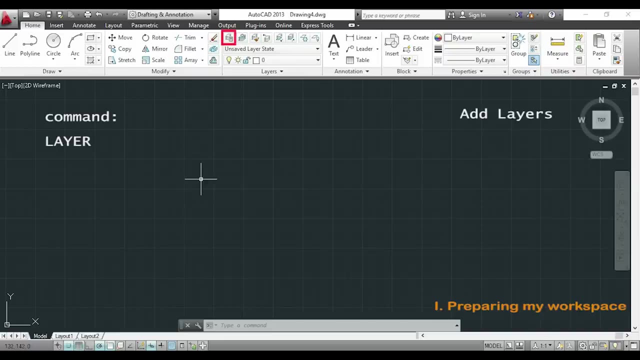 So the next thing is to set up my layers. If you pay attention to the drawing, you will notice that I have different colors here, and that's because I separate in layers the doors, the windows and the walls To create a new layer. I can type layer with my keyboard or clicking this button here. 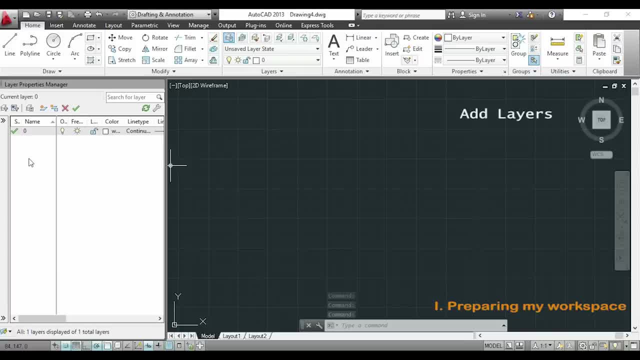 This is the layer properties manager. To add a new layer, just click somewhere in this box with the right button And now I will click on new layer. So for my first layer, I will name it as walls, And I will do the same for all the other layers. 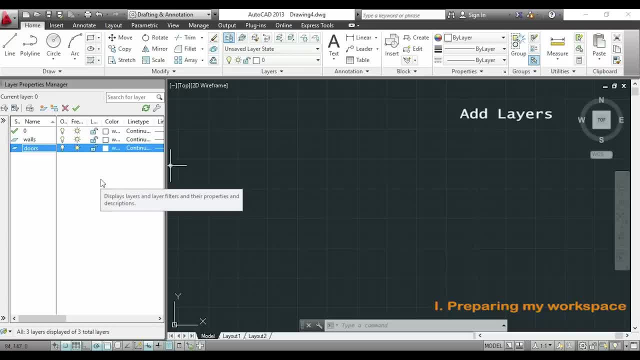 The second one, I will name it as doors, This one windows, And the last one will be the dimensions for the dimension lines. Now I will change the colors for all my layers And I will change the colors for all my layers. 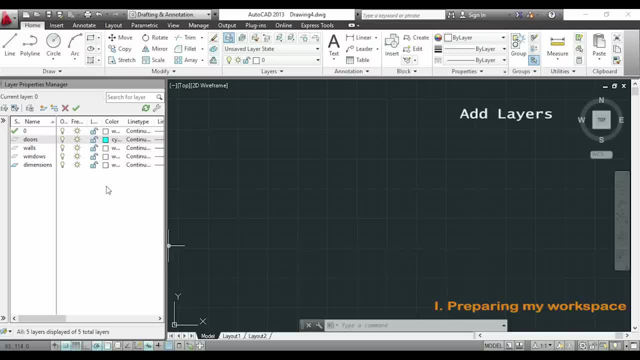 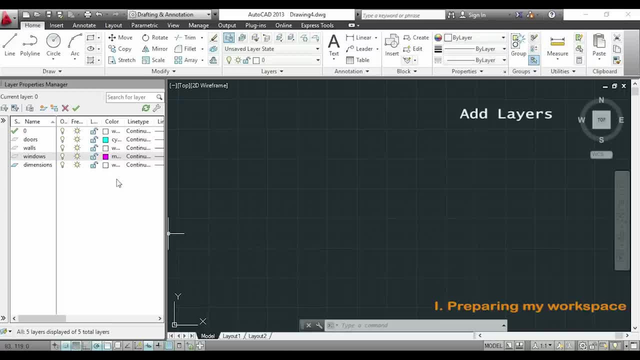 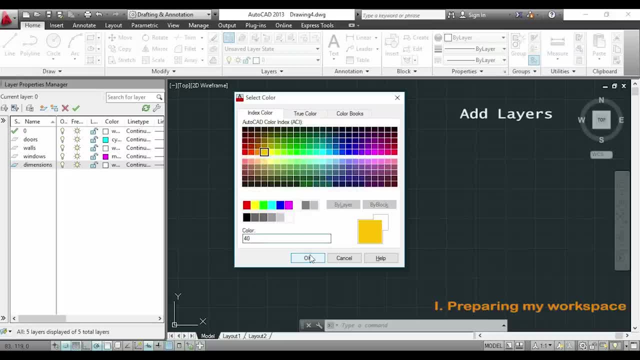 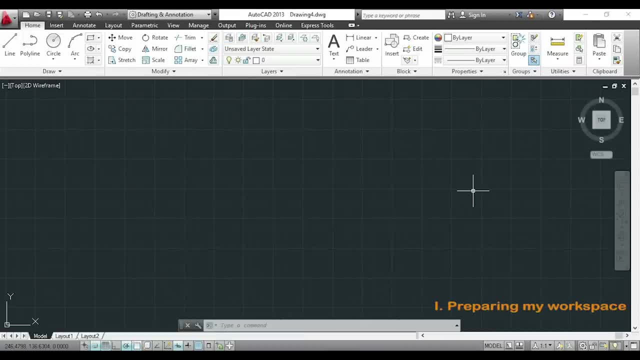 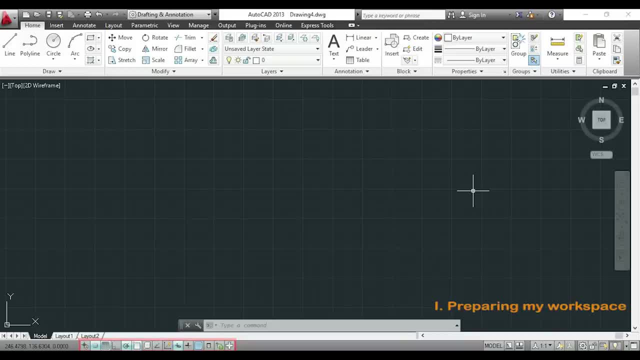 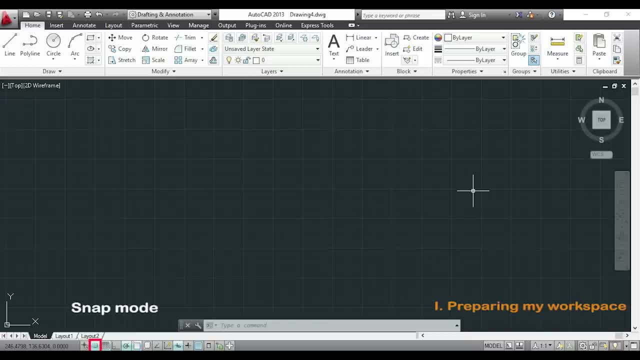 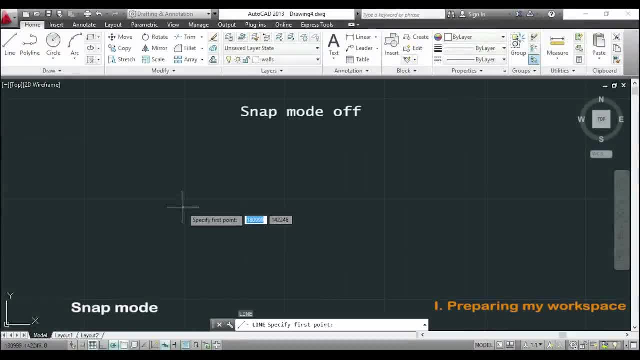 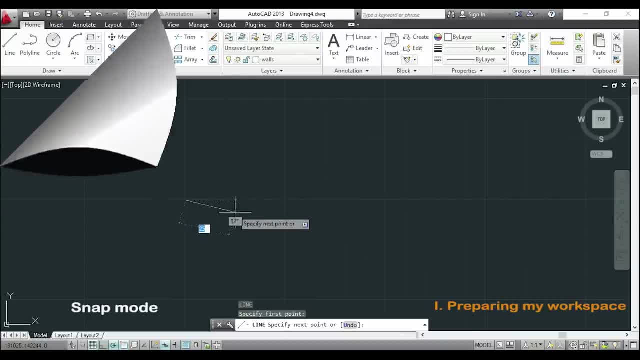 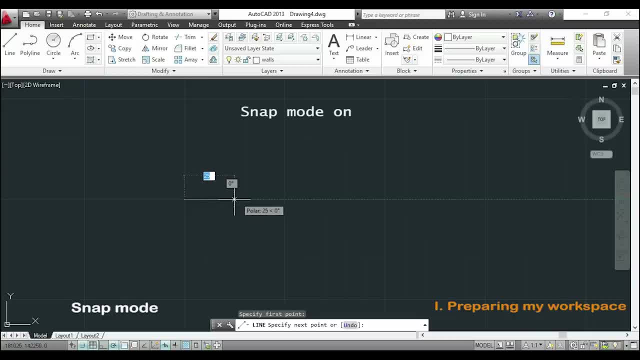 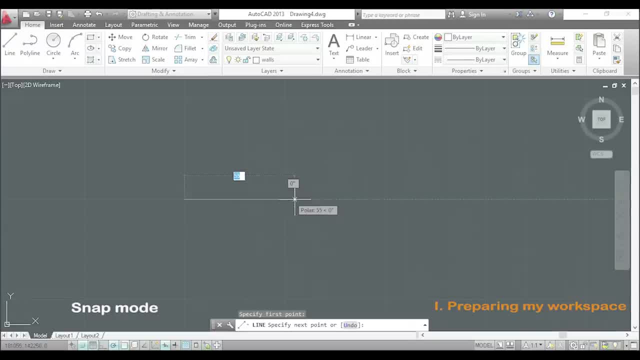 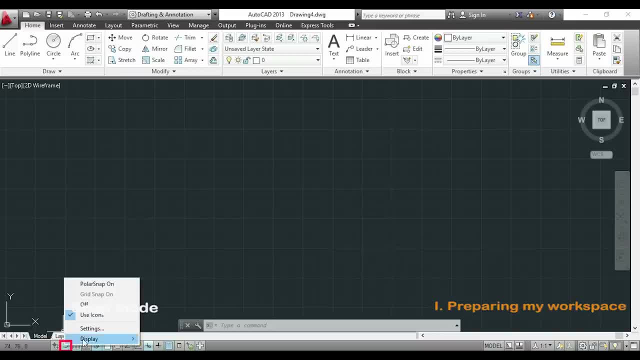 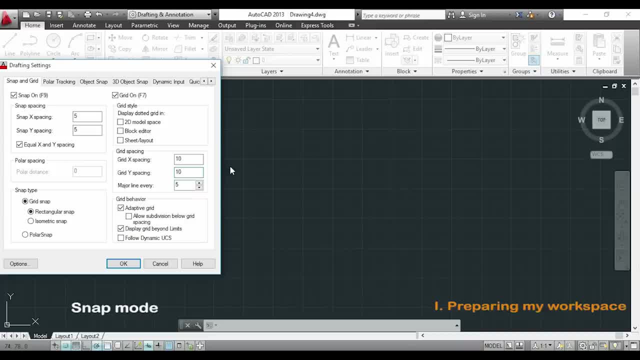 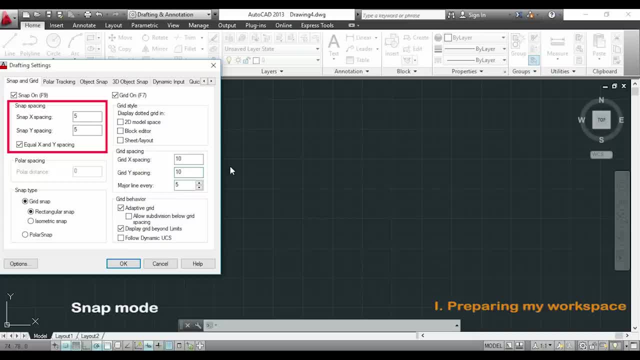 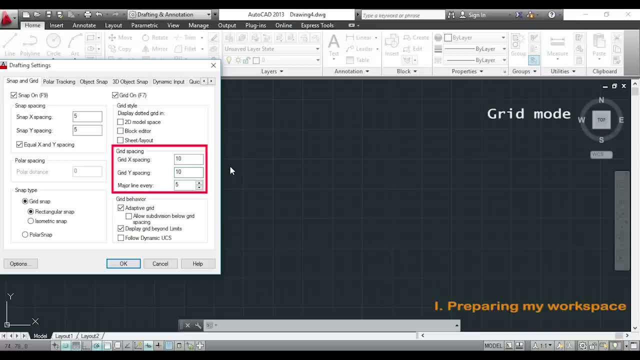 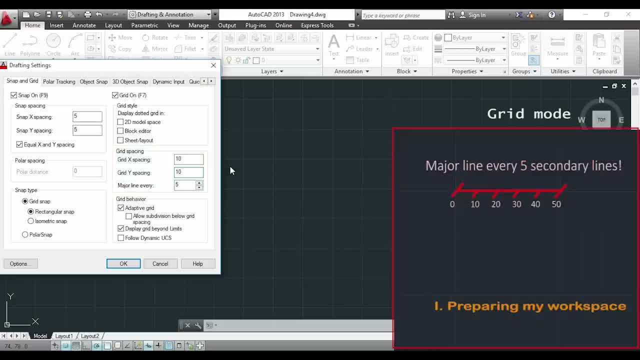 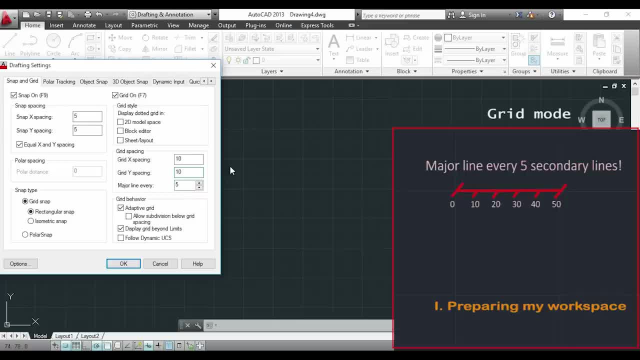 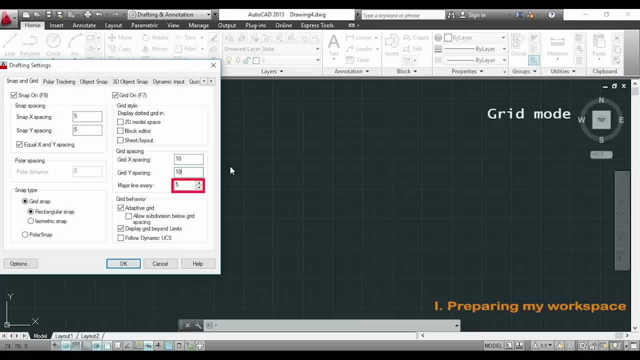 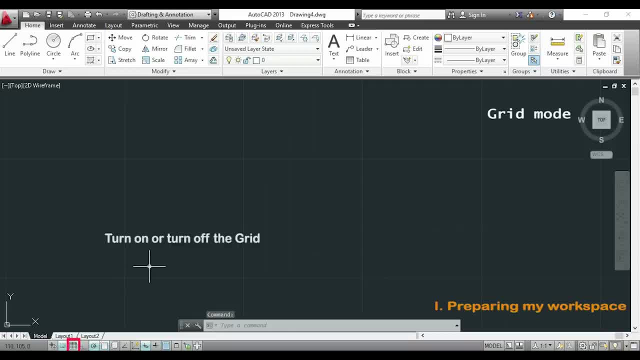 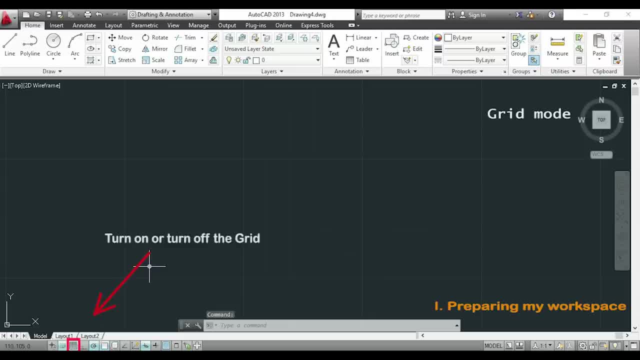 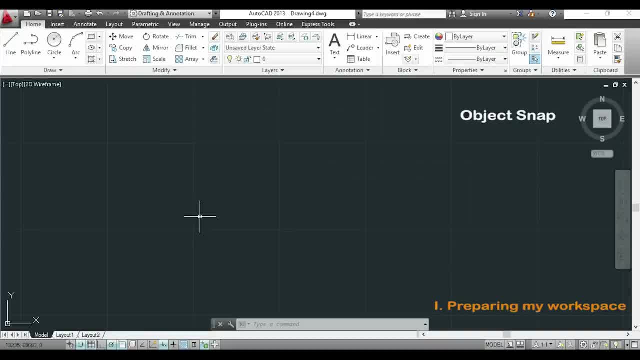 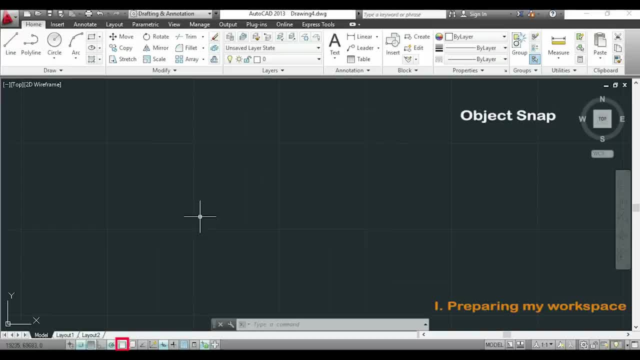 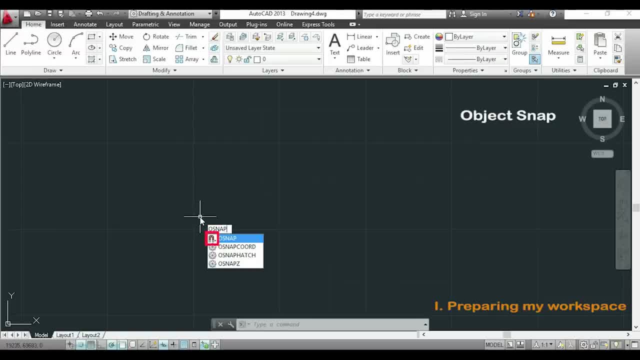 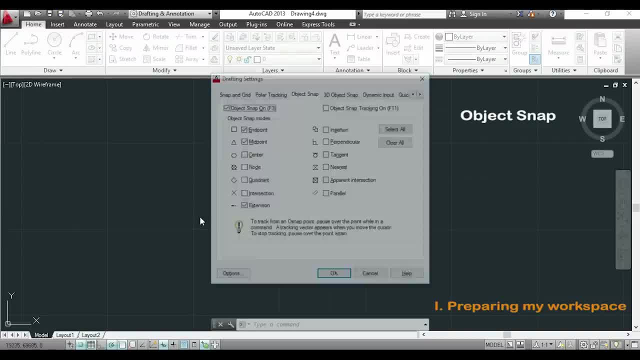 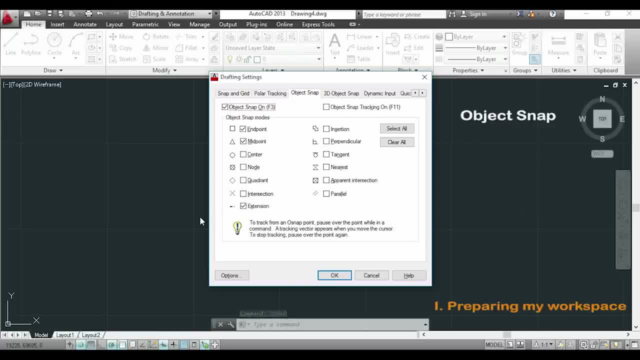 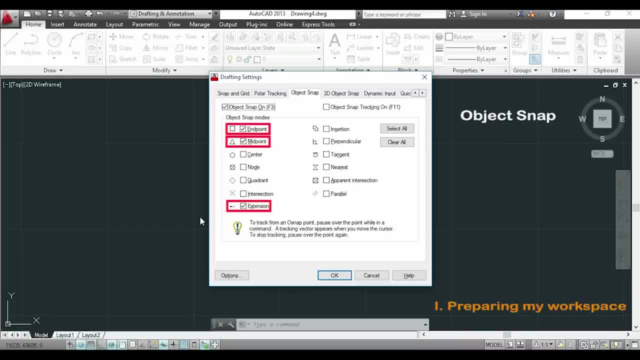 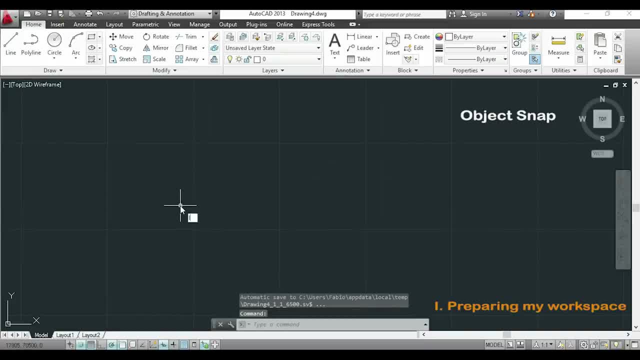 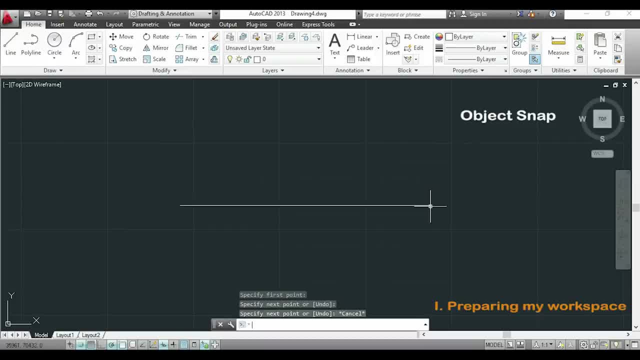 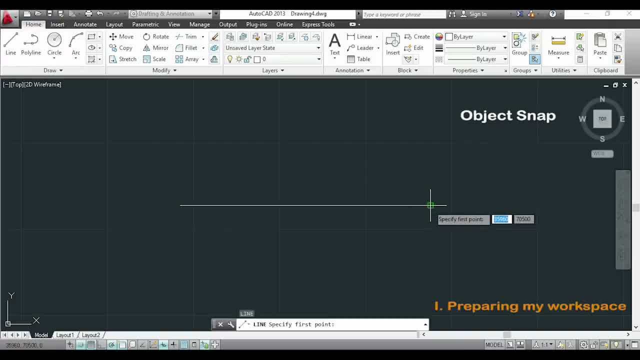 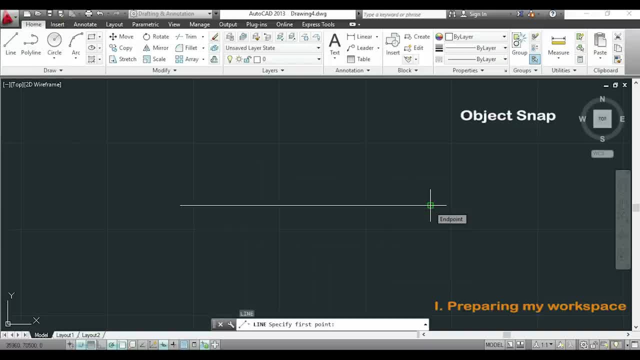 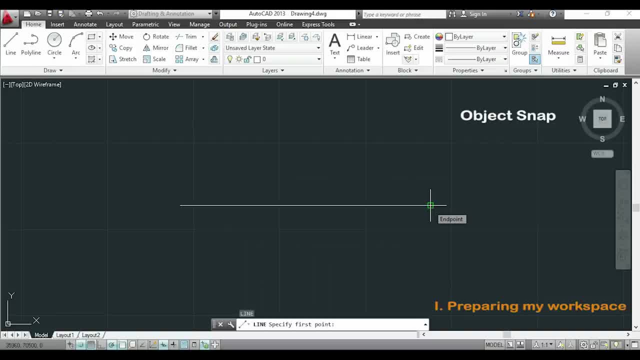 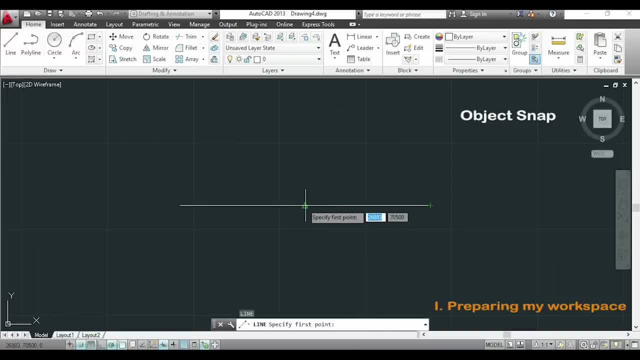 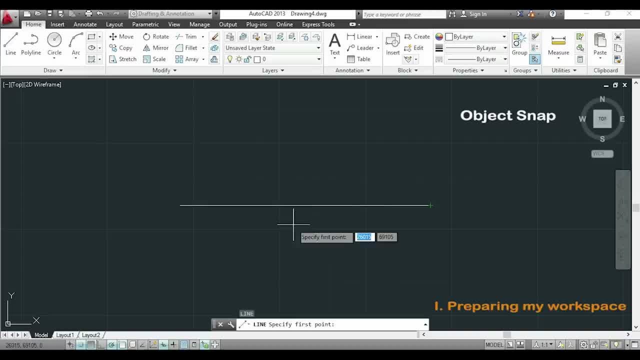 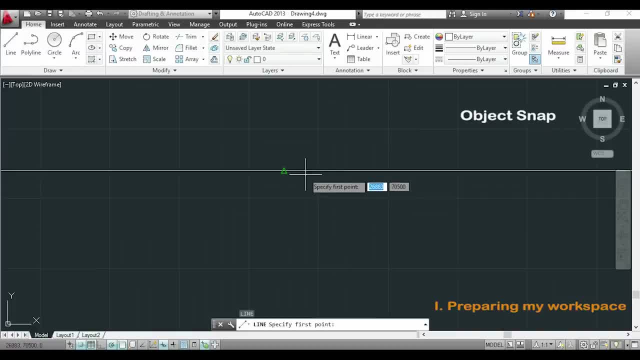 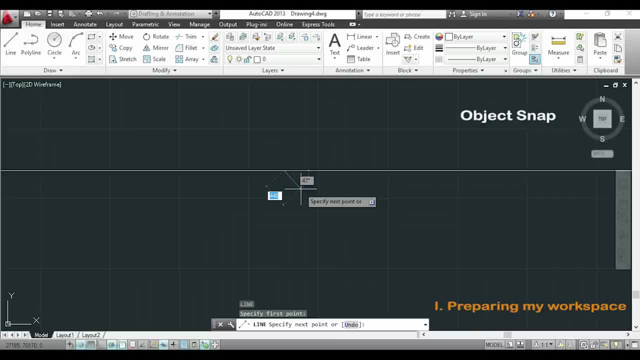 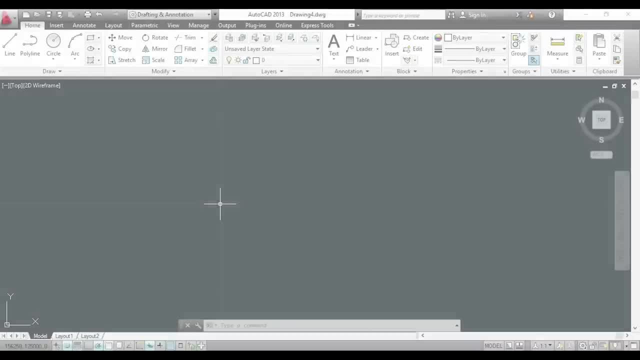 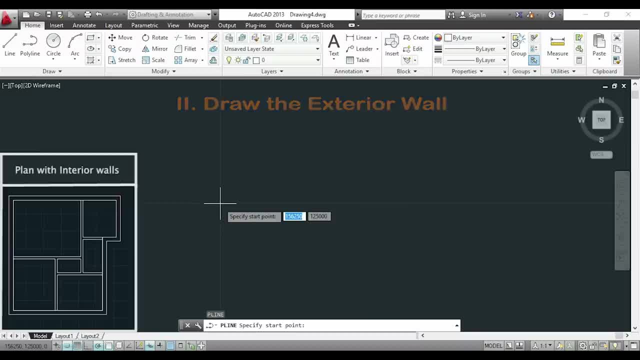 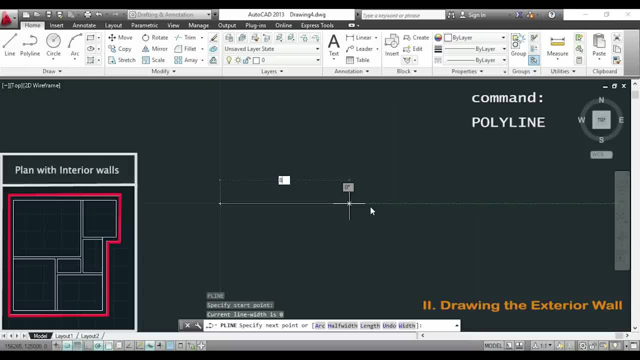 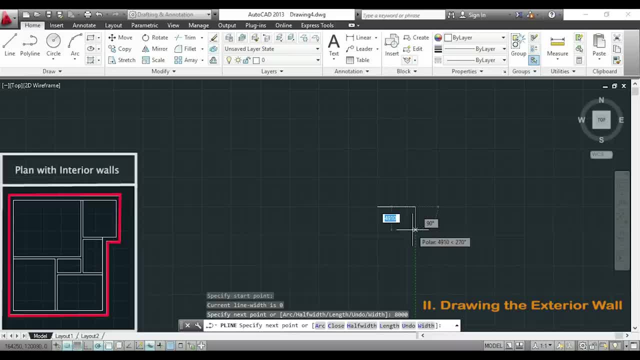 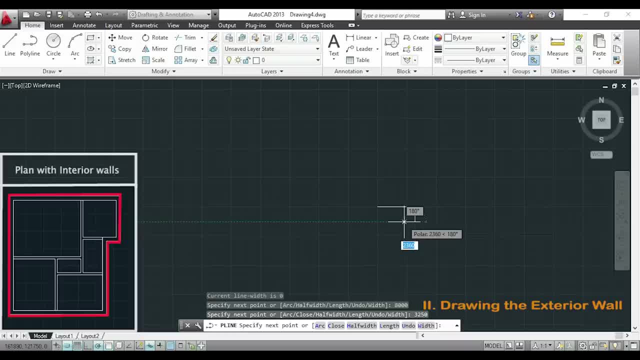 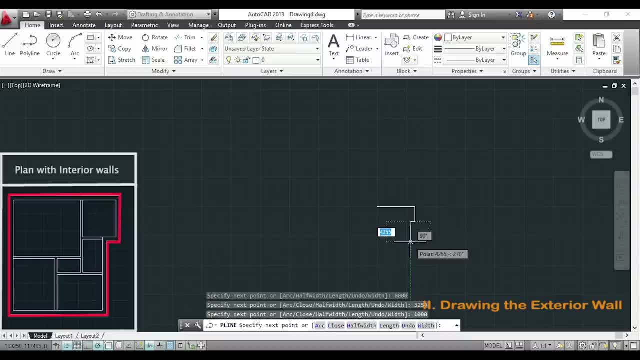 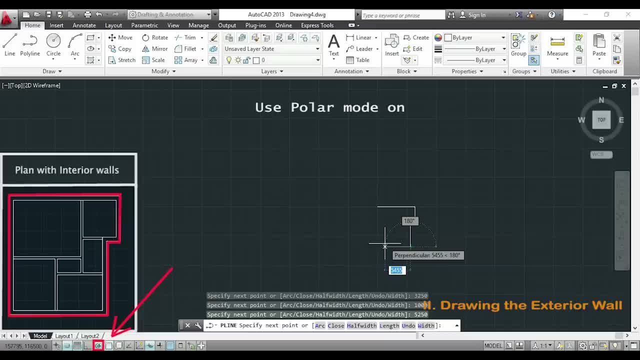 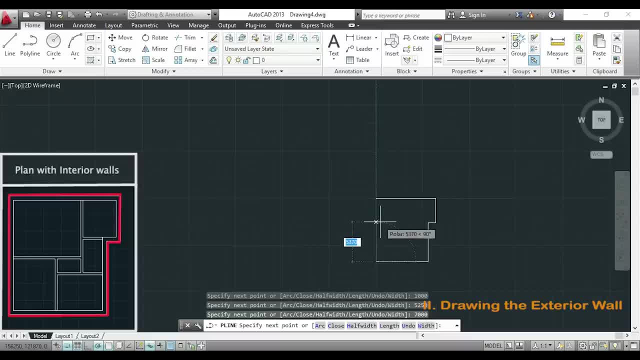 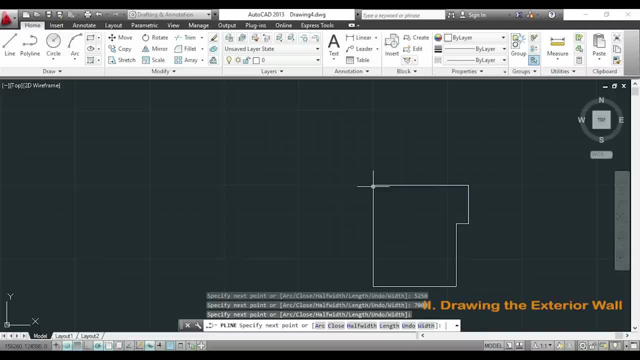 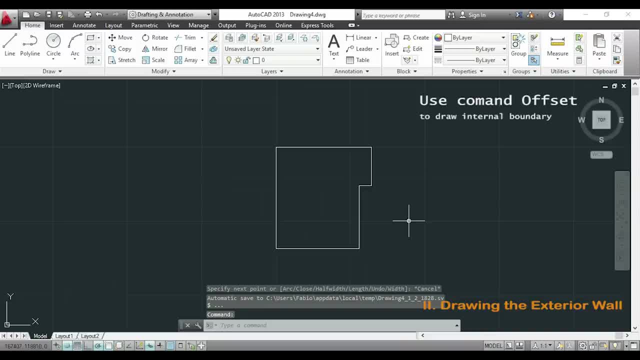 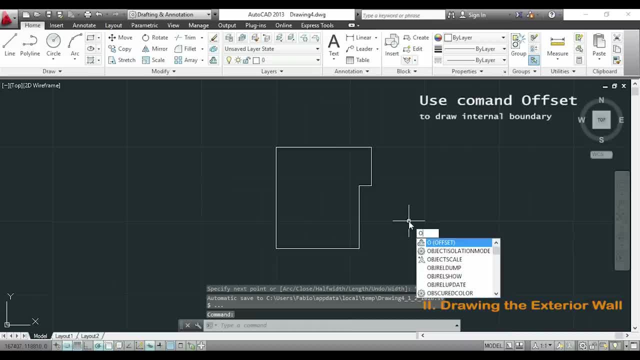 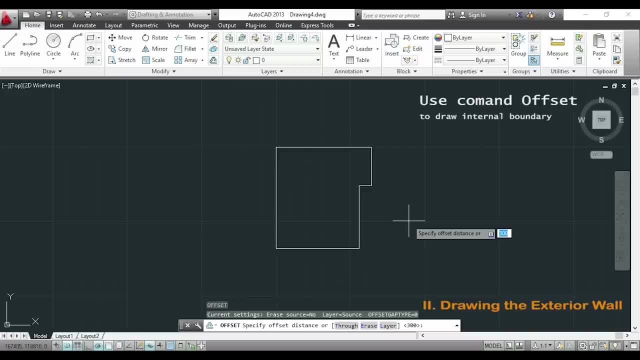 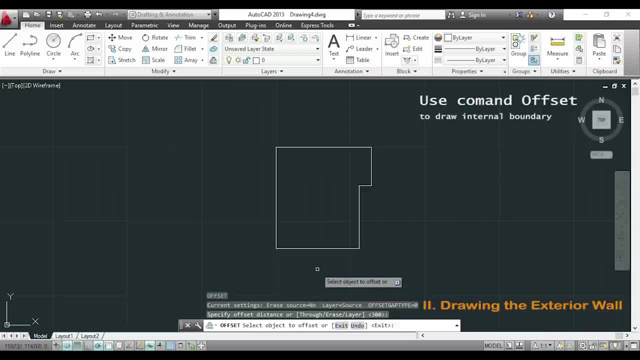 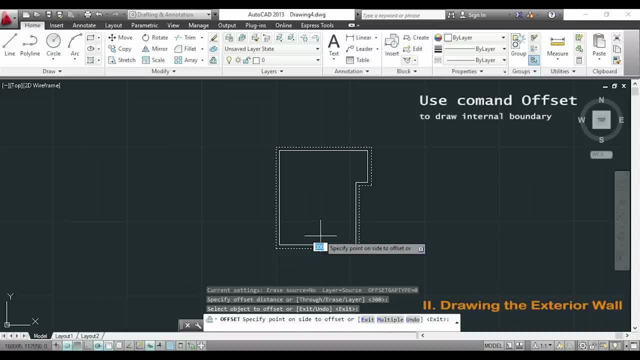 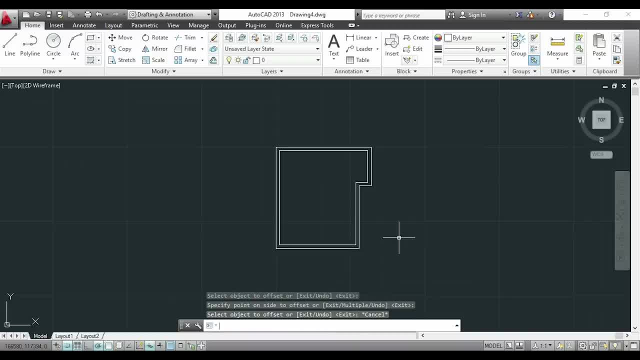 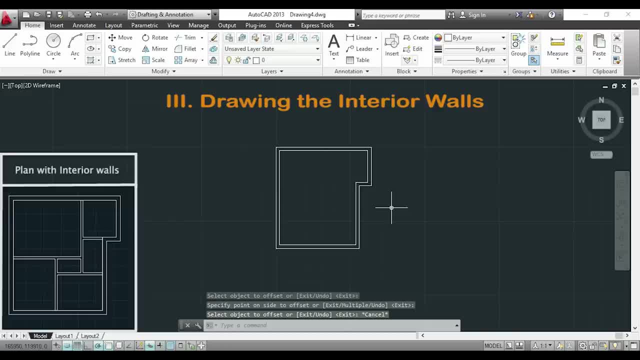 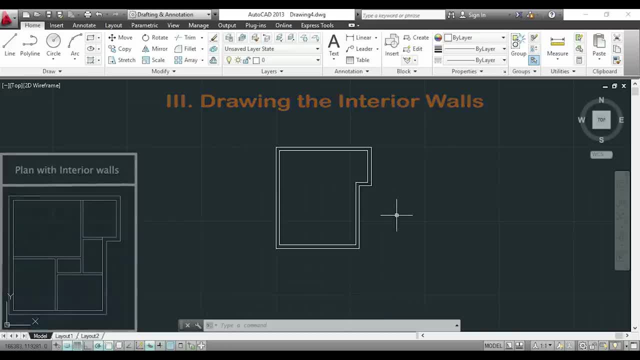 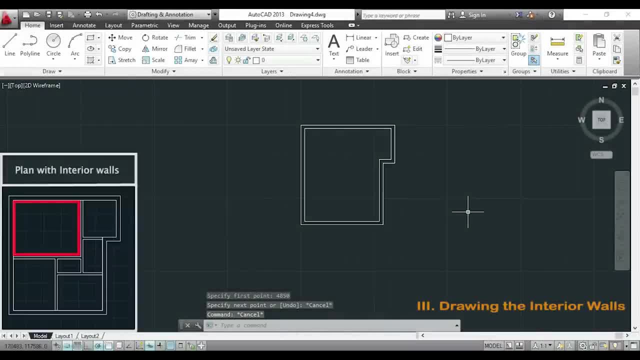 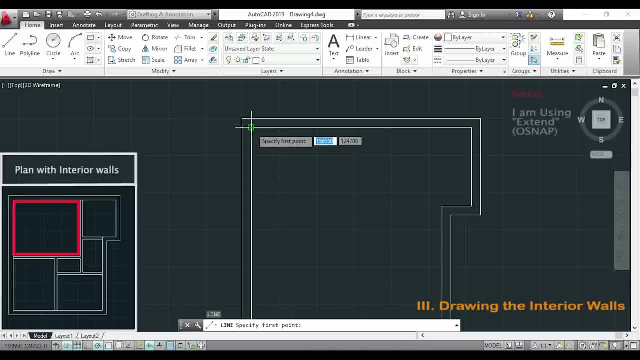 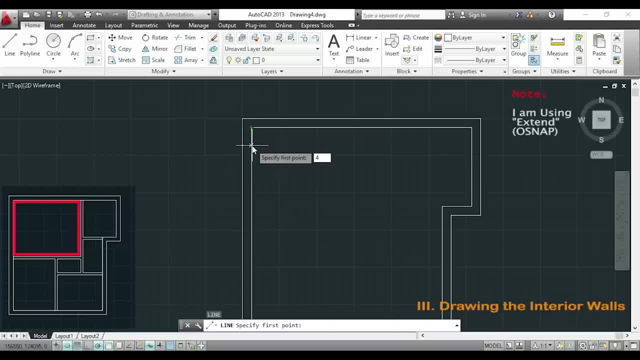 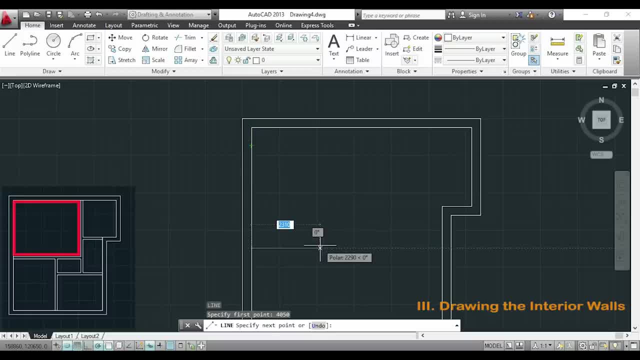 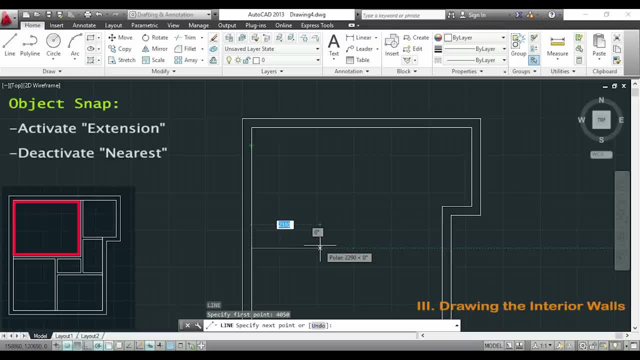 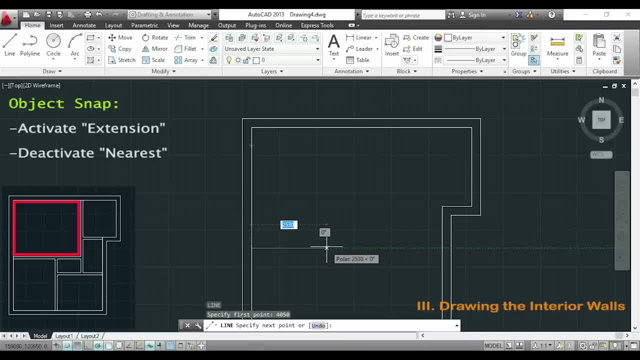 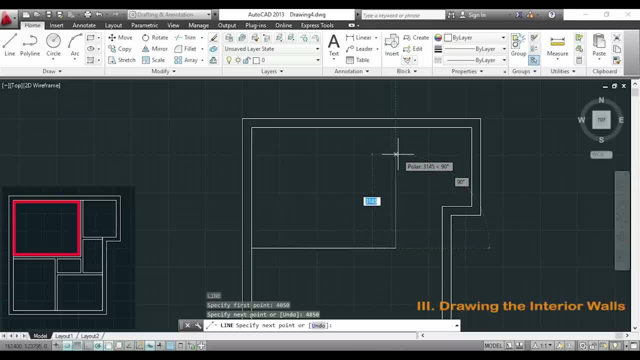 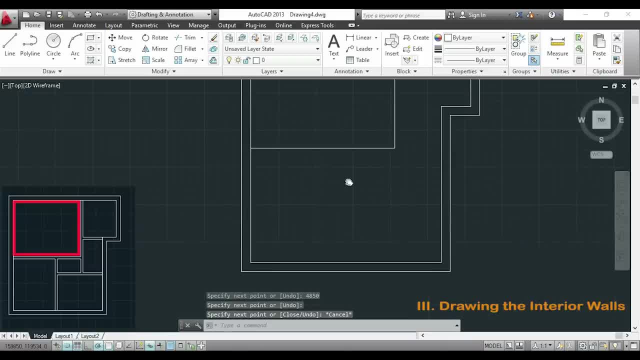 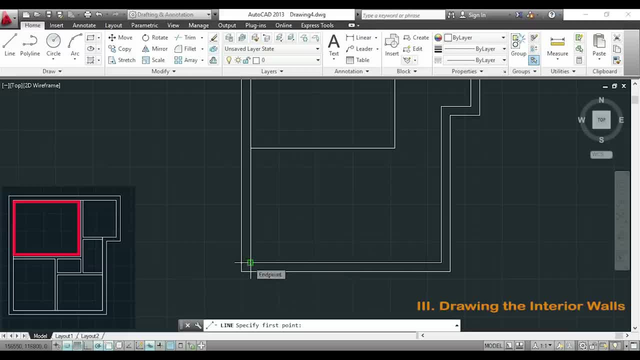 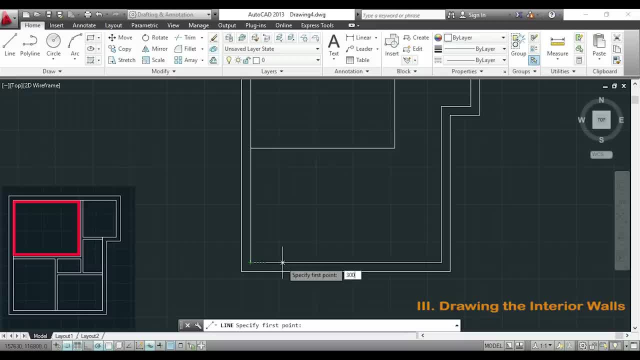 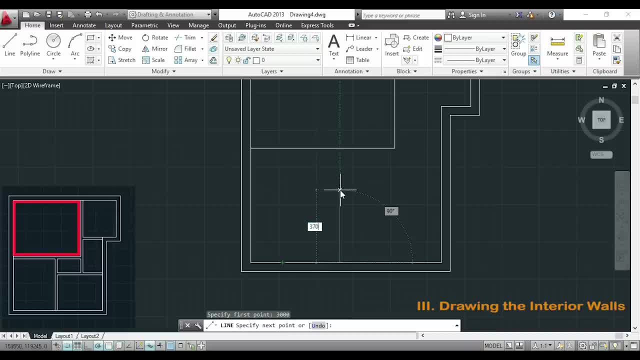 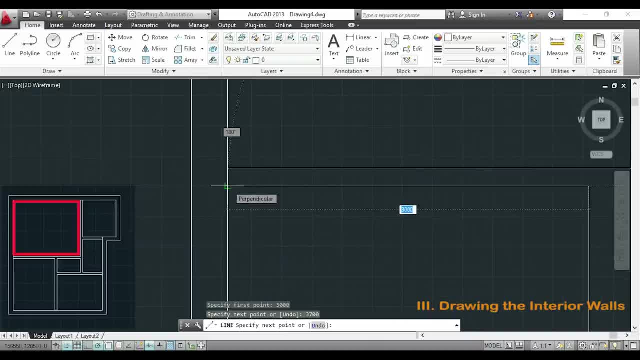 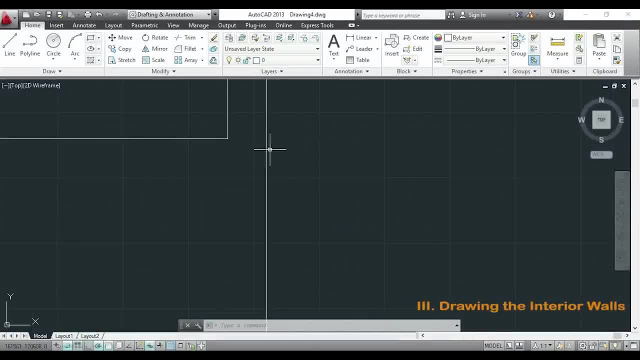 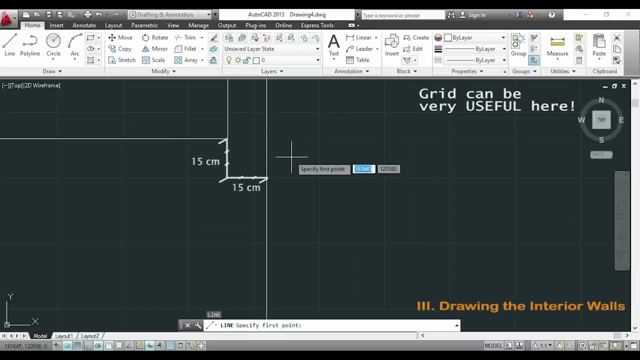 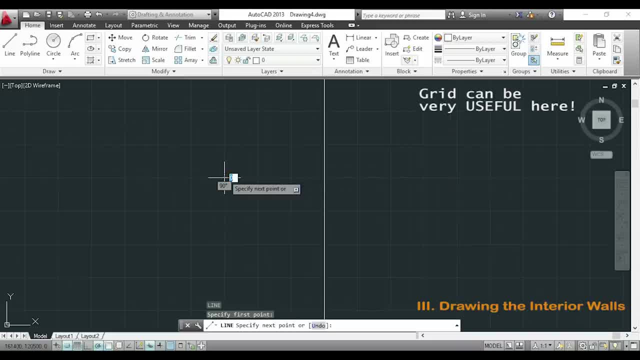 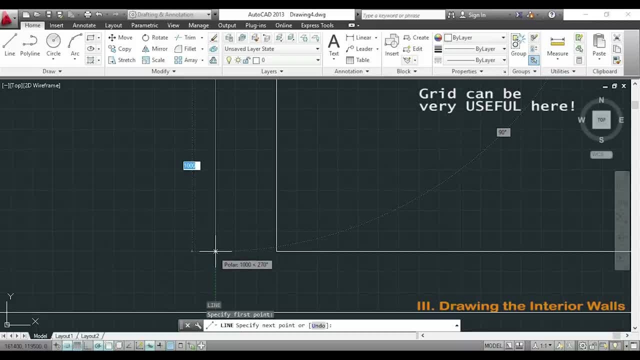 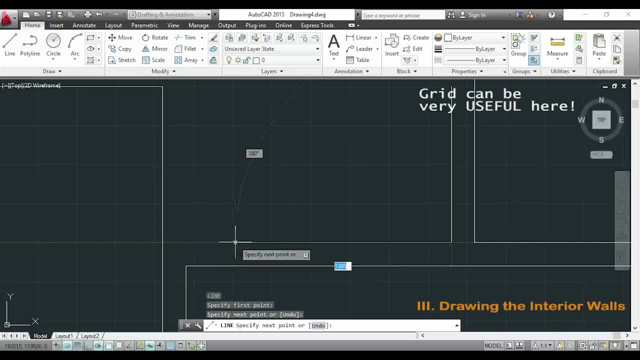 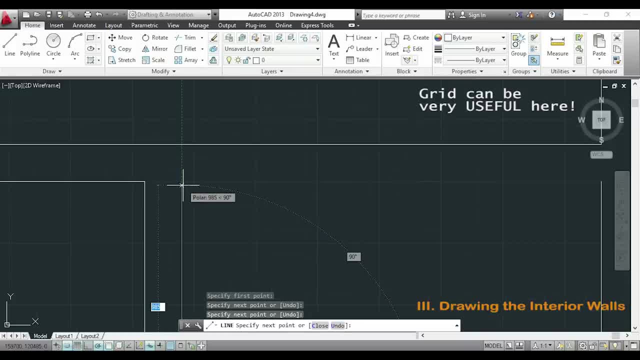 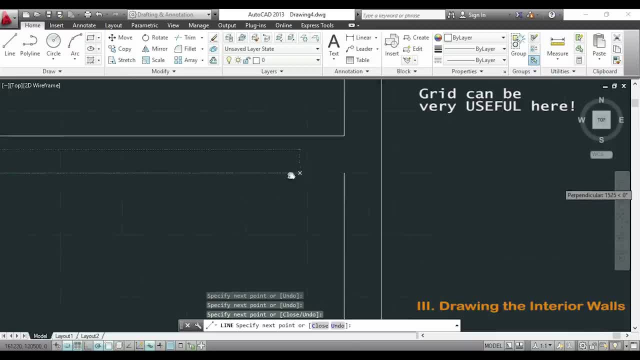 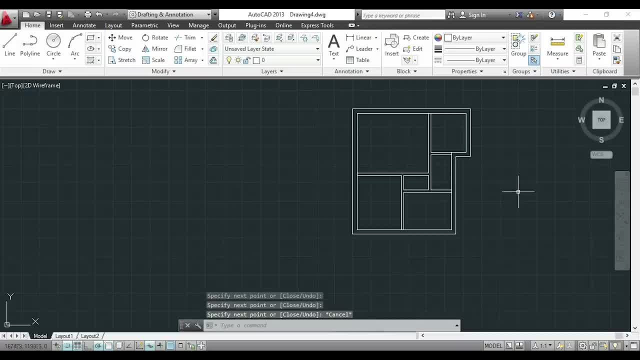 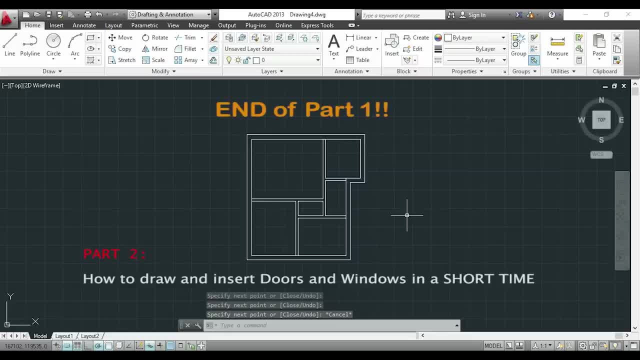 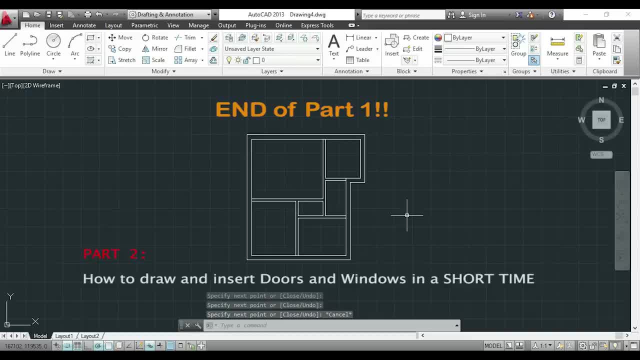 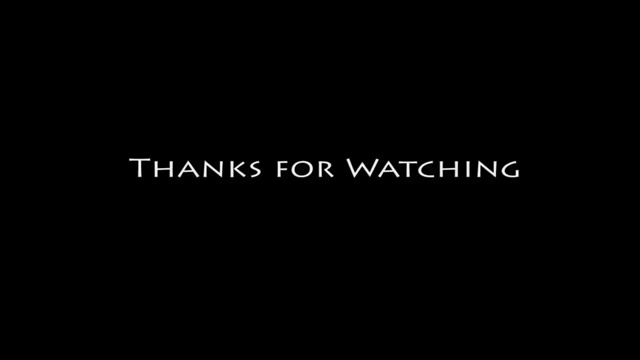